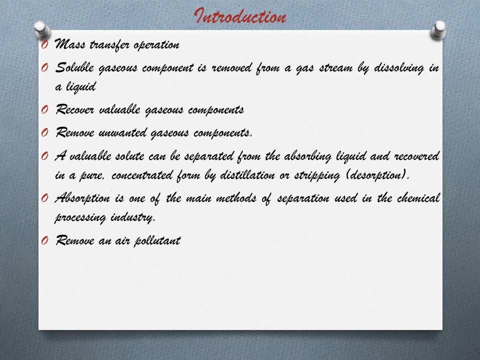 A well-reliable solute can be separated from the absorbing liquid and recovered in a pure, concentrated form by distillation or stripping. It is one of the main methods of separation. It is used in the chemical processing industry: Accompanied biochemical reaction between the absorbed component and the reagent in the absorbing fluid. 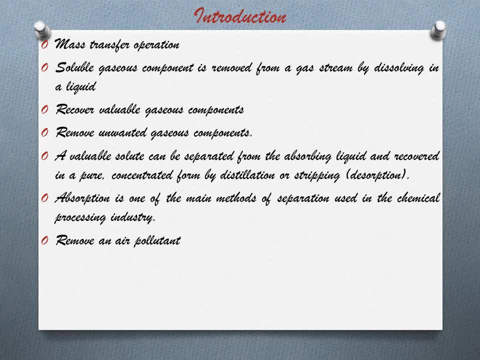 absorption can become a very effective means of separation. Absorption can also be used to remove an air pollutant, like an acid gas, from the stream. Then system could be a simple absorption in which the absorbing liquid is used in a single process, used in a single path and then disposed of while containing the absorbed pollutant. 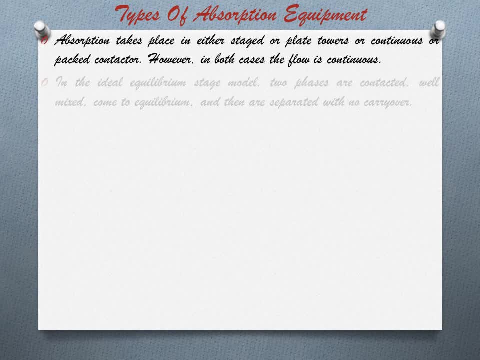 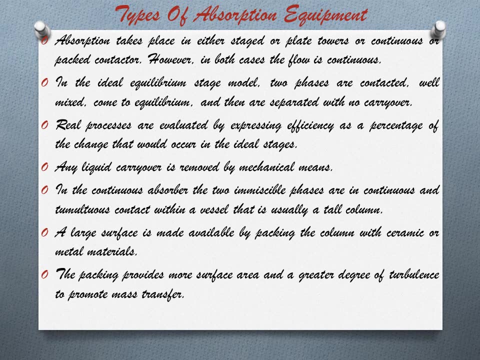 Next we discuss about various equipments used for absorption. Absorption takes place in either stage or plate towers, or continuous or packed contents. However, in both cases the flow is continuous. In the ideal equilibrium stage models, two phases are contacted well-mixed, come to equilibrium and then are separated with no carryover. 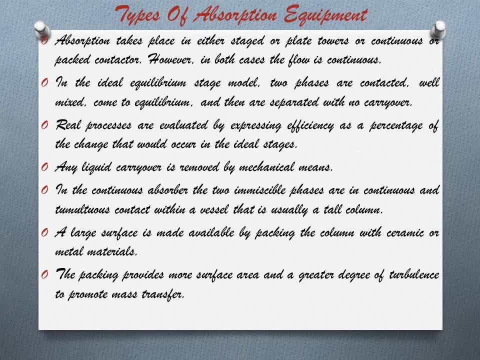 Real processes are evaluated by expressing efficiency as a percentage of the change that would occur in the ideal stages. Any liquid carryover is removed by mechanical means. In the continuous absorption, the two immiscible phases are in continuous and stimulative contact within a vessel that is usually a tall column. 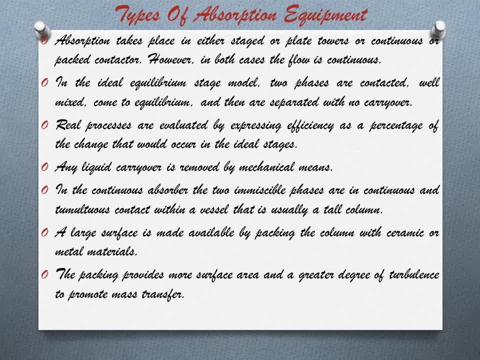 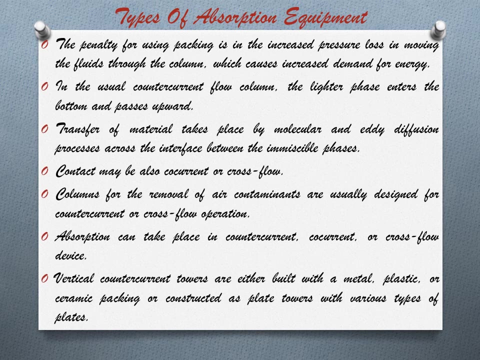 A large surface is made available by packing the column with ceramic or metal material. The packing provides more surface area and a greater degree of turbulence to promote mass transfer. The difficulty for using packing is in the increased pressure loss in moving the fluids through the column, which causes an increased demand for energy. 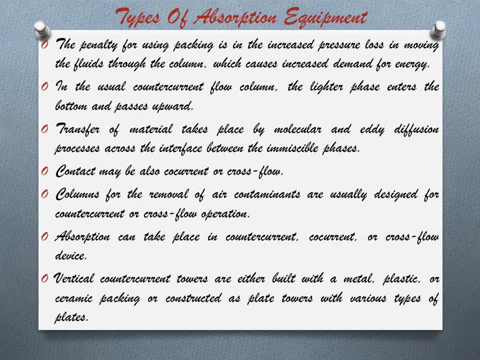 In the usual countercurrent flow column, the lighter phase enters the bottom and passes upwards. Transformed material takes place by molecular and eddy diffusion processes across the interface between the immiscible phases. Transformed material takes place by molecular and eddy diffusion processes across the interface between the immiscible phases. 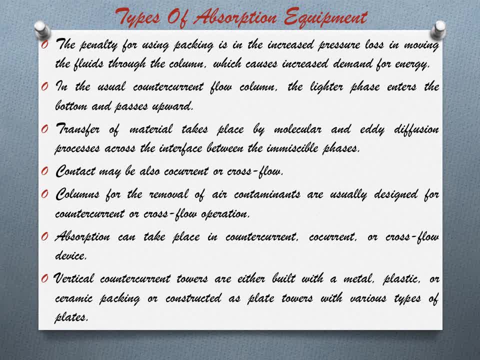 Contact may be also co-current or cross-flow. BLM 933 Columns for the removal of air contaminants are usually designed for counter current or cross-flow operation. Absorption can take place in a counter current, co-current or cross flow device. Vertical counter current towers are either built with a metal, plastic or ceramic packing. 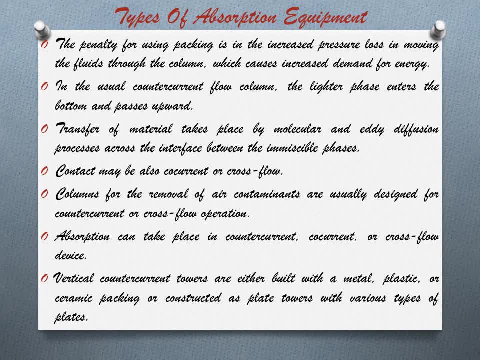 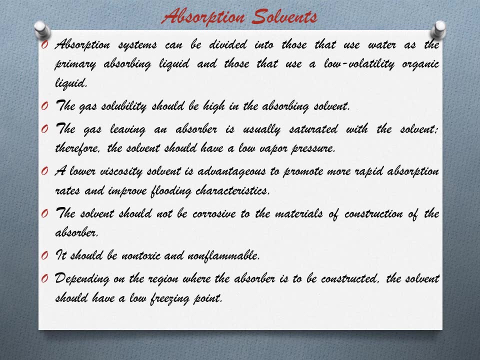 or constructed to support the coloured surface, or constructed as plate towers with various types of plates. Now we will discuss about the absorption solvents. Absorption systems can be divided into those that use water as the primary absorbing liquid and those that use a low-volatility organic liquid. 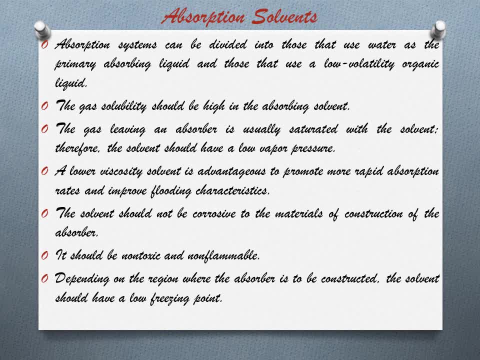 The gas solubility should be high in the absorbing solvent. The gas leaving an absorber is usually saturated with the solvent. Therefore the solvent should have a low vapour pressure. A lower viscosity solvent is advantageous to promote more rapid absorption rate and improve flooding characteristics. 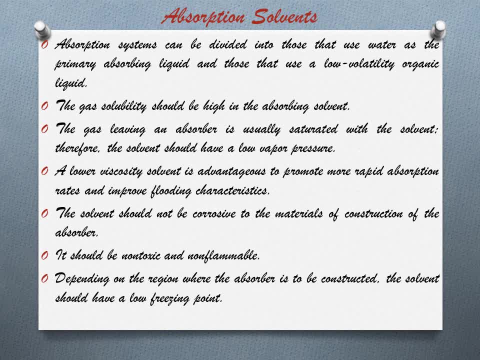 The solvent should not be corrosive to the material of construction of the absorber. It should be non-toxic And non-flammable. Depending on the reason where the absorber is to be constructed, the solvent should have a low facing point. 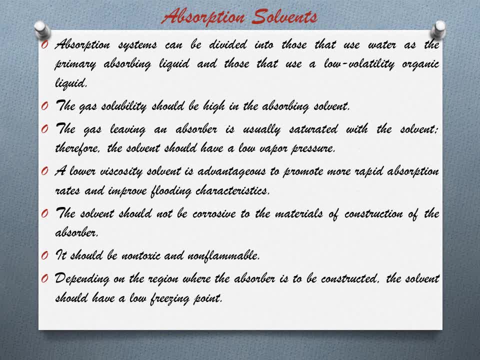 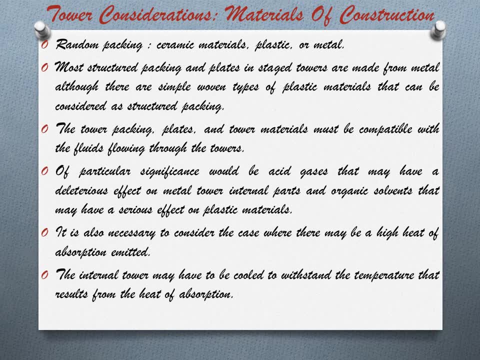 Now we will discuss about the material construction. Random packing can be made from ceramic materials, plastic or metal. Most structured packing and plates in stage towers are made from metal, Although there are simple movement types of plastic materials that can be considered as structured packing. 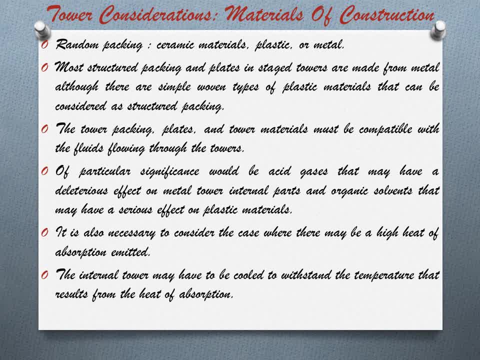 The tower, packing plates and tower materials must be compatible with the fluid flowing through the tower. Of particular significance would be acid gases that may have a deleterious effect on metal tower internal parts and organic solvents that may have a serious effect on plastic materials. 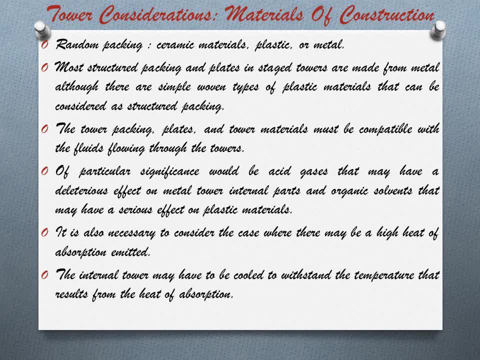 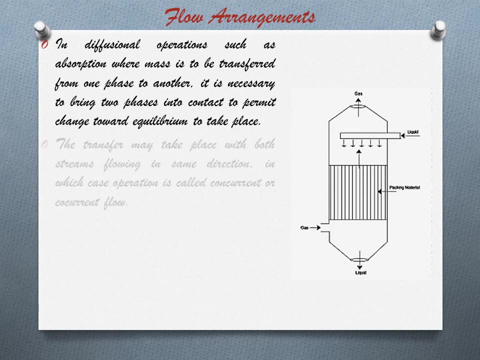 It is also necessary to consider the case where there may be a high heat of absorption emitted. The internal tower may have to be cooled to withstand the temperature that results from the heat of absorption. Now we will discuss various flow arrangements in absorption column. In diffusional operations such as absorption, where mass is to be transferred from one phase to another. 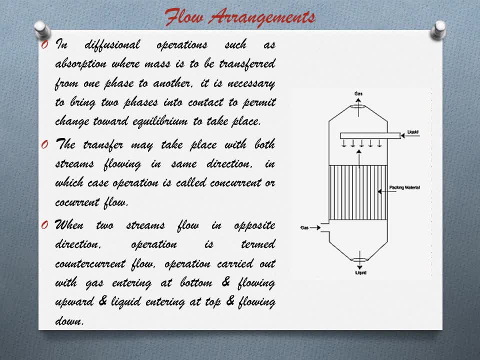 it is necessary to bring the two phases into contact to permit the change toward equilibrium to take place. The transfer may take place with both streams flowing in the same direction, in which case the operation is called co-current flow, When the two streams flow in the opposite direction. 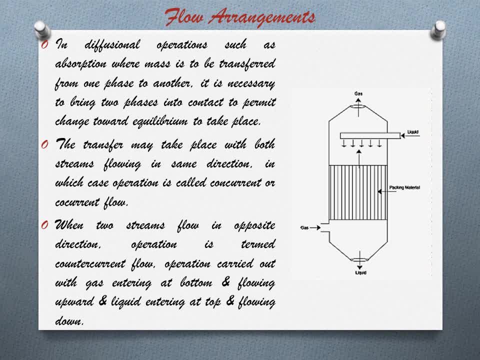 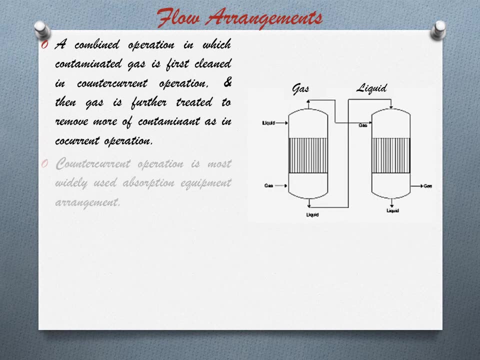 the operation is termed as counter-current flow, An operation carried out with the gas entering at the bottom and flowing upward, and the liquid entering at the top and flowing down. This process is shown in the figure Now: a combined operation in which the contaminated gas is first fleeing in a counter-current operation. 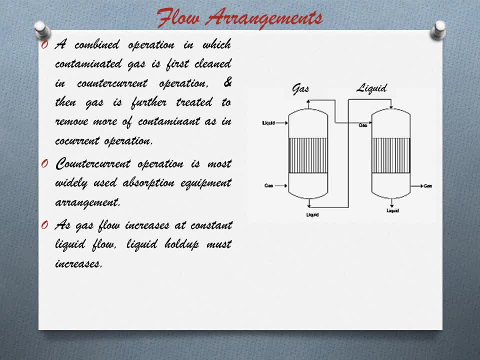 and then the gas is further treated to remove more of the contaminant, as shown in the counter-current flow. This is the counter-current operation that follows. Counter-current operation is the most widely used absorption equipment arrangement. As the gas flow increases at constant liquid flow, liquid holdup must increase. 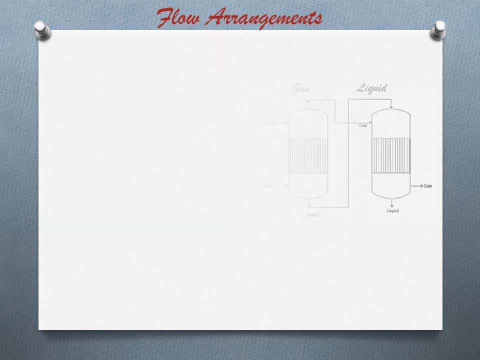 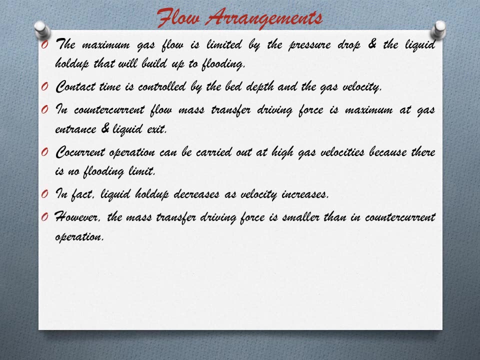 The maximum gas flow is limited by the pressure drop and the liquid holdup that will build up to flooding. Contact time is controlled by the bed depth and the gas velocity In counter-current flow. mass transfer driving force is maximum at the gas entrance and liquid exit. 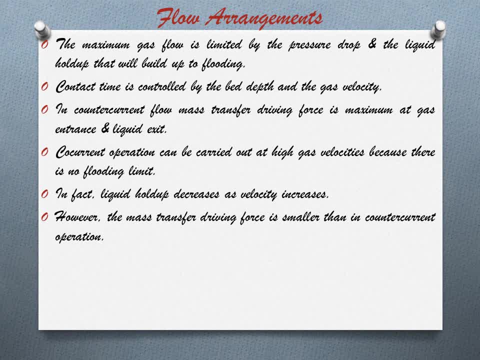 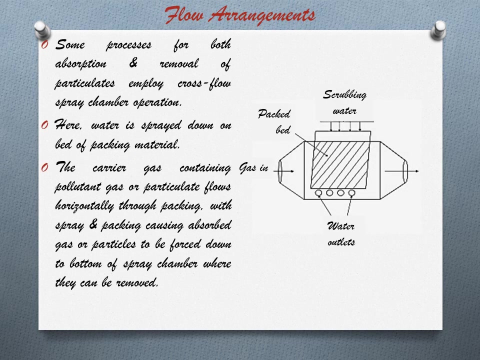 Co-current operation can be carried out at high gas velocity because there is no flooding limit. In fact, liquid holdup decreases as velocity increases. However, the mass transfer driving force is smaller than in counter-current operation. Some processes for both absorption and the removal of particles imply a cross-flow spray chamber operation.